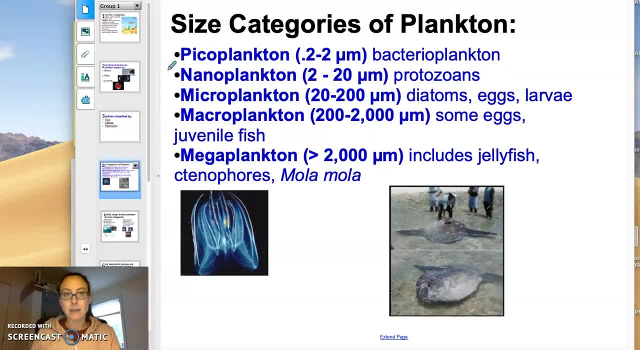 So let's start with size. Tiny picoplankton are maybe up to two whole microns micrometers in size. So these are bacteria. Bacteria in the plankton are really important because they're going to be breaking down dead material. So these are the decomposers. 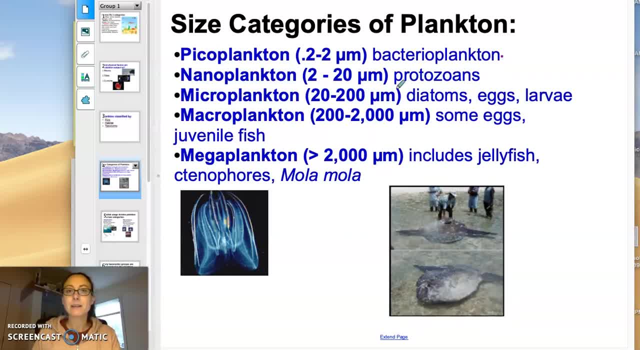 They may also do photosynthesis. The next big, bigger size is up to 20 whole nan, Yeah, micrometers, And these are called nanoplankton. They're protozoan, So single cell, very small Still on the mostly single-celled side of things are microplankton. 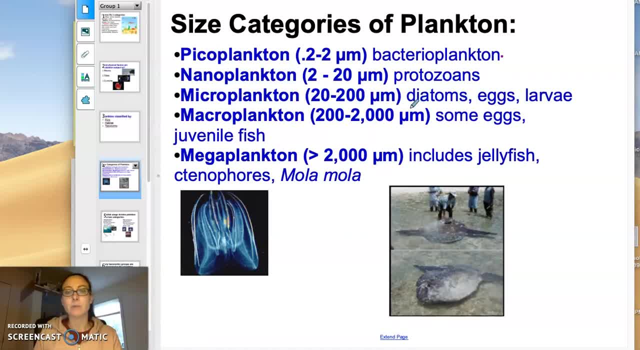 So we're going to learn about diatoms because they're very, very important to the marine ecosystem. We'll also see that the eggs of certain fish and other living organisms, animals fit into this category, And some larvae, so the babies of certain species. 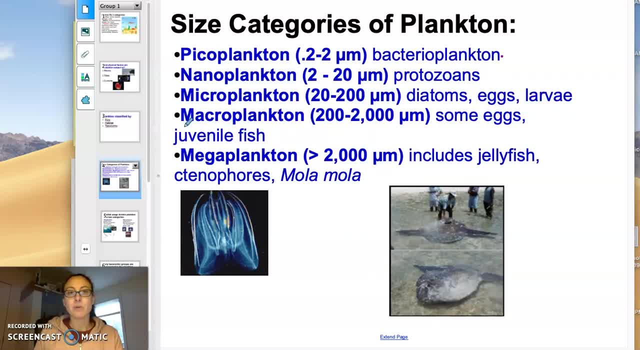 Macro. So what we might think of as large is still like maybe two centimeters in size. So 2000 microns is about two centimeters. We're talking again fish, larvae and eggs and things like that On the gigantic, gigantic side of plankton. 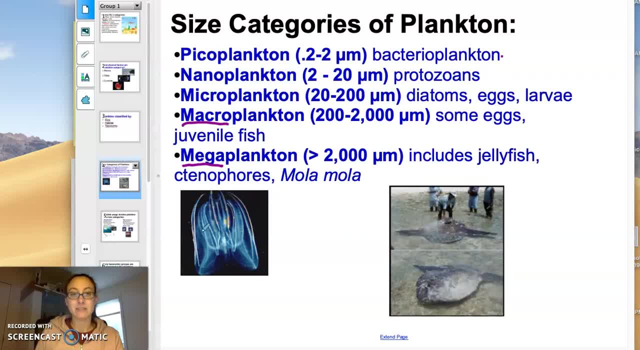 we have things that are as gigantic as this tinafore, comb, jelly, and even the mola mola- which is a fish that really can't swim And so it's technically considered plankton- and those can get up to like six to eight feet long. 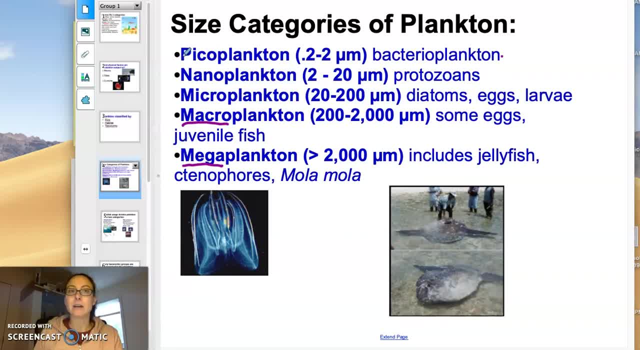 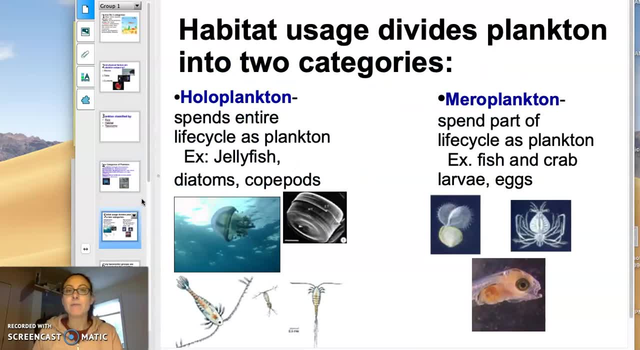 So there's really a huge range in size, from bacteria all the way up to these mega plankton. So if we were to look at categories based on how they use the space in terms of their lifespan, we have organisms called hollow plankton, meaning these are species that live their entire life in the water. 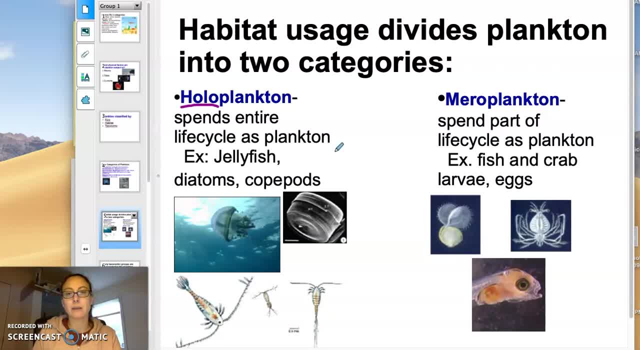 and can never really swim against current and can never really join the benthos. So, jellyfish, And this is a scanty fish, This is a scanning electron micrograph, So really zoomed in, of a diatom And this is what copepods really look like as seen under the microscope. 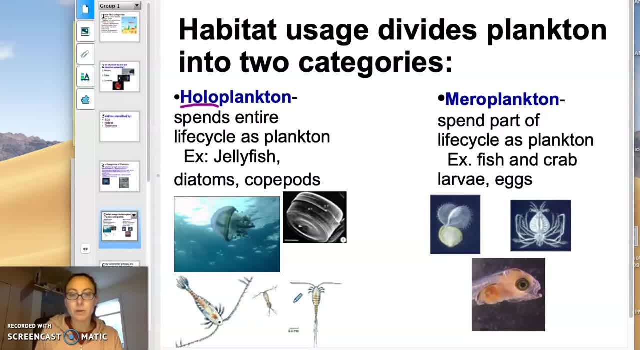 This is a sketch, but that's their actual appearance. For those of you who think SpongeBob is accurate, All right. On the other side of things, there are species that only live part of their lifespan in the plankton, So things like crabs and snails and fish are going to, as adults, live on the bottom benthic organisms. 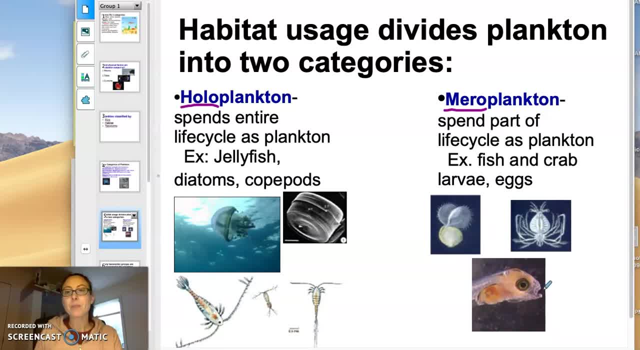 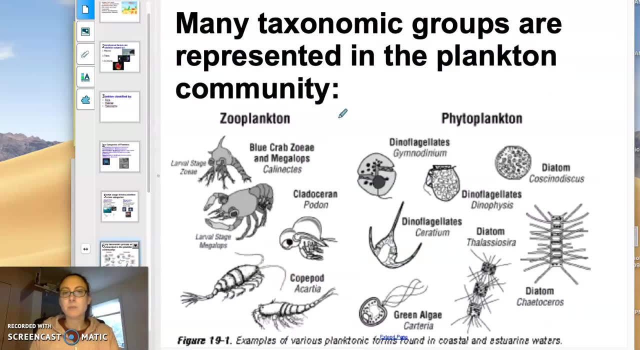 or be able to swim against the current as necton, But when they're juveniles, they're pushed around by the currents. They really can't do anything about that. So, finally, we're going to look at the different groups of types of species. 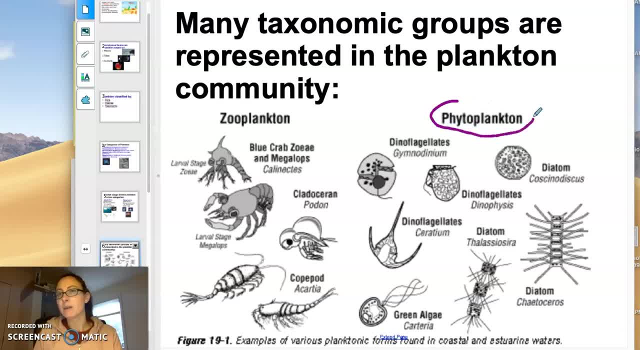 The two big groupings are phytoplankton- These are the plant like plankton that do photosynthesis, And we'll get into a couple of these different types here. And the zooplankton- ZOO is the prefix, that means animal. 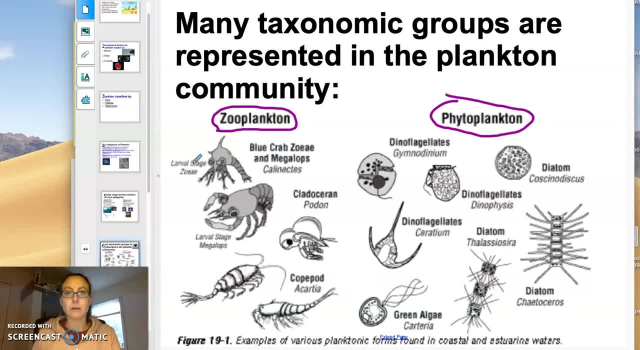 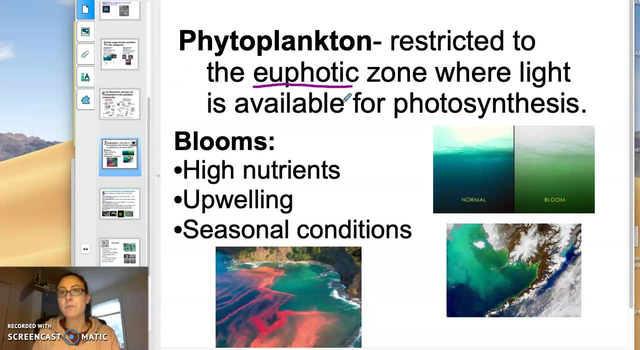 So all the animal kingdom plankton. So let's start with some of those phytoplankton. Thing to know about phytoplankton. Remember they have to do photosynthesis, So they have to be in the euphotic zone and they need nutrients. 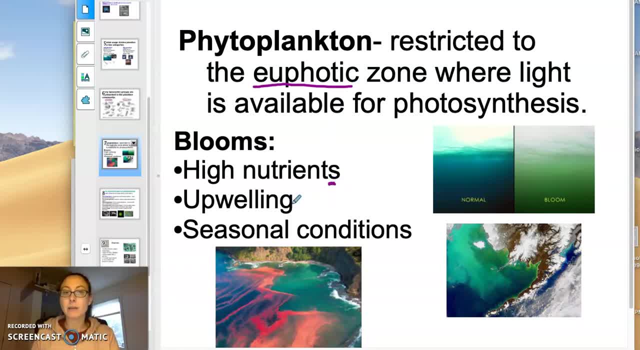 So if we have a place where there is an upwelling, or seasonal currents bring nutrients, or maybe rain that causes nutrients to come off the shore, we are going to get something called a phytoplankton bloom. That means lots and lots of these tiny phytoplankton are growing and reproducing. 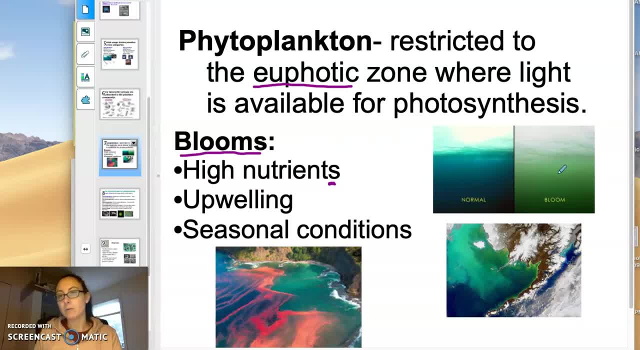 So that normally blue water would become green with their abundance, And so we can see satellite images. So this is off the coast of Alaska. This is as temperatures warm up and sunlight becomes available. We get phytoplankton blooms in this region. 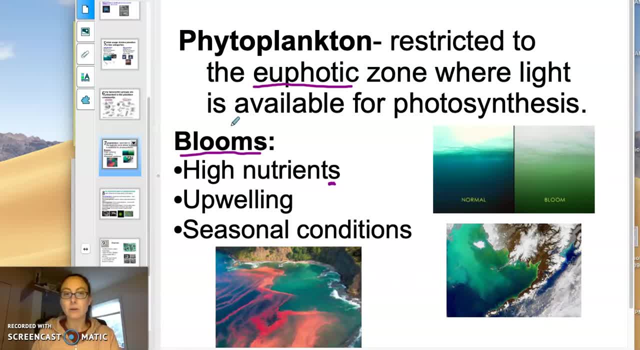 So that would be in the summertime. We can also have phytoplankton blooms of phytoplankton that are not green, And so this is a red tide That is caused by certain types of phytoplankton becoming very common due to rain event. 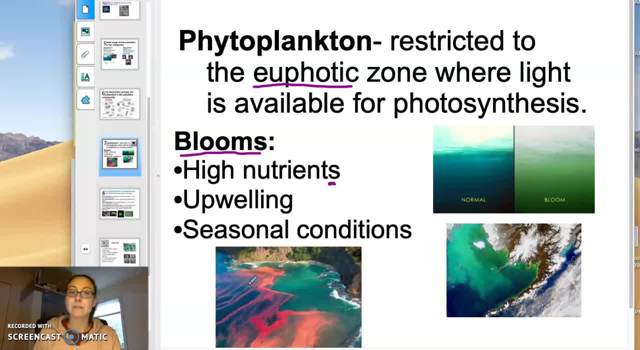 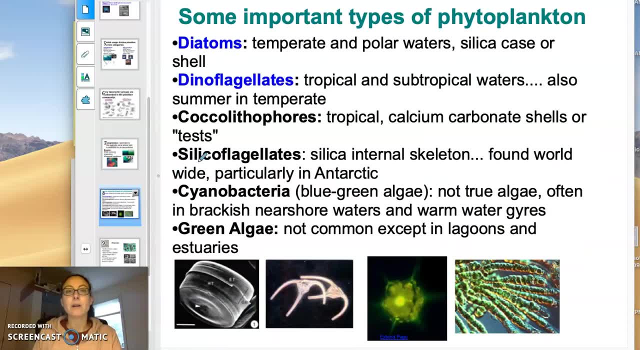 pushing up lots of nutrients offshore, And that's not something you want to get caught out in And we'll talk about that in a moment. So there are a lot of different groups. This is not a fully biological oceanography course, So you're not going to have to know all about these different ones down here. 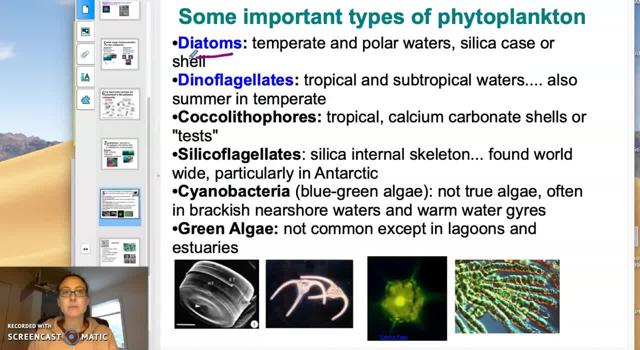 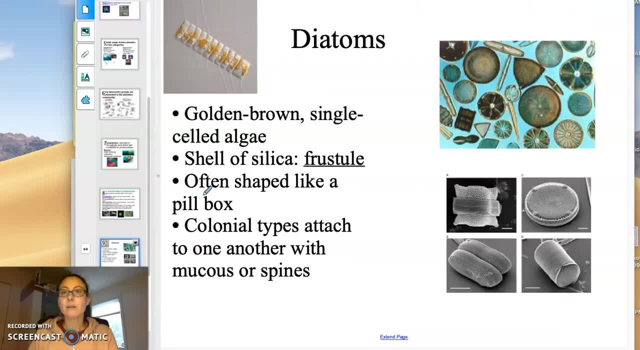 But two big groups You should know about are diatoms and dinoflagellates, because they're very, very abundant and very important. Diatoms are sometimes referred to as being a pillbox shape, because they have a hard shell made of silica. 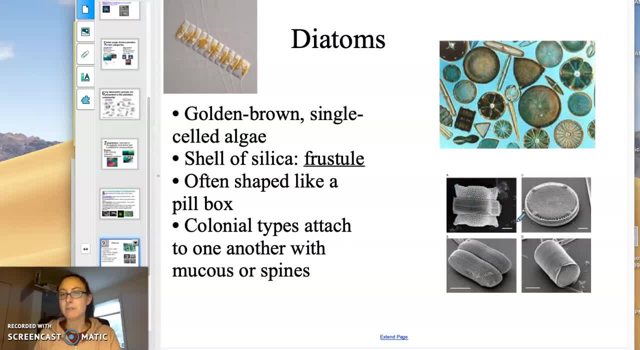 And they have a top half and a bottom half that fit together kind of like a little tin box or something like that, And so they reproduce by that population. So they do that by that popping apart, and each half becomes the half of a new one. 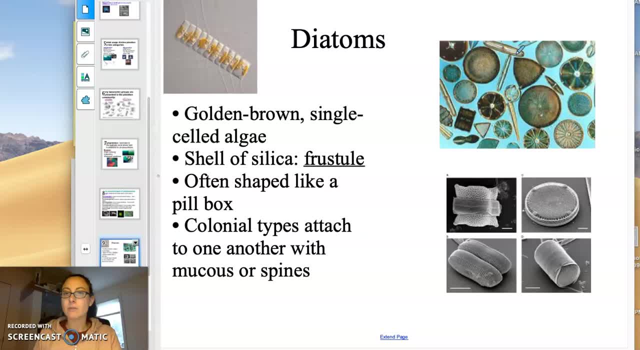 They can live individually on their own and get lots of different shapes and sizes, Or this: you can see this has some spines, They're growing and that helps them make long chains. So we would call that being colonial, meaning part of a colony. 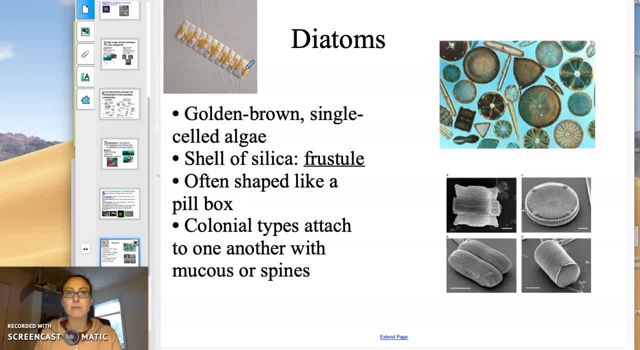 The pigments that they use for photosynthesis are, for example, are a golden brown color, and so diatoms are what cause a lot of the rocks in the area to look kind of like they've got a brown slime on them. You might sometimes 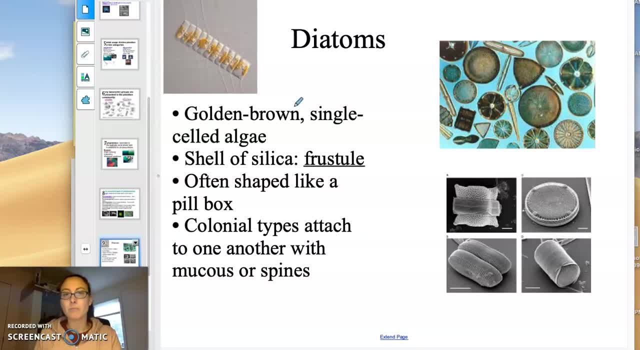 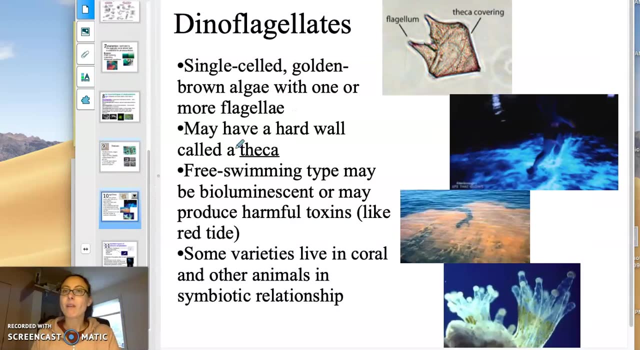 see algae that has sort of a fluffy brownish tinge to it. That's probably because they're covered in diatoms and very, very abundant in ecosystems like Sipicant Harbor. Dinoflagellates are a different group. These ones have a 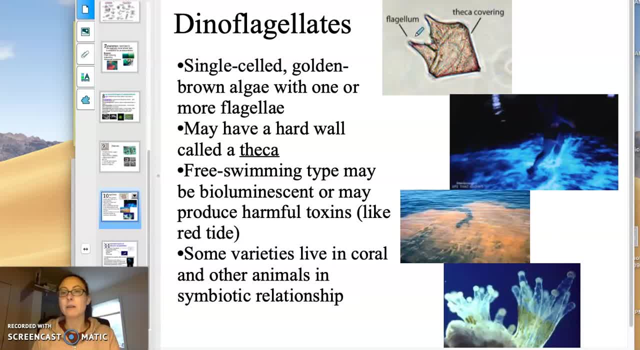 flagellum, so hopefully you learned about that in biology. They can swim around a tiny bit. Their shell is made out of carbohydrates and other types of material. that makes it not quite as hard but but a little bit more flexible. Again, these are mostly golden brown in color, but sometimes they can make a more orangy or 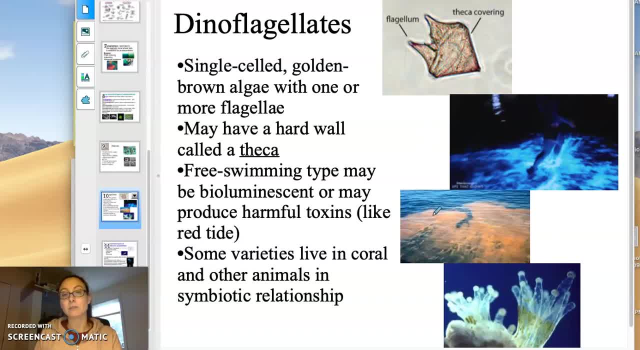 red color. So dinoflagellates- certain species- are the ones that produce harmful toxins and make something like red tide, which is one example of a harmful algal bloom. These, these dinoflagellates, will produce toxins that are irritating for skin and 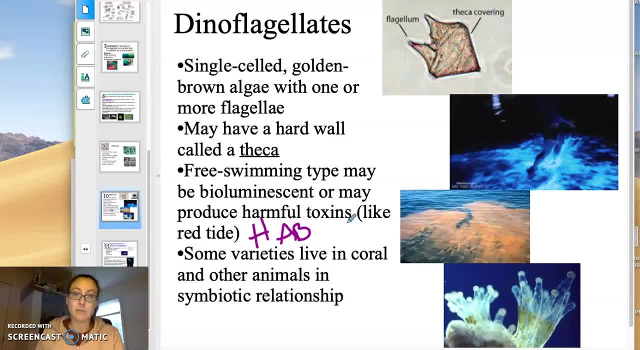 if we were to eat shellfish that ate those diatoms by filtering them out of the water, we would get very sick, And that's what causes certain shell fisheries to close for a while until they process the toxins out of them. A nicer example of dinoflagellate are the groups that are bioluminescent. 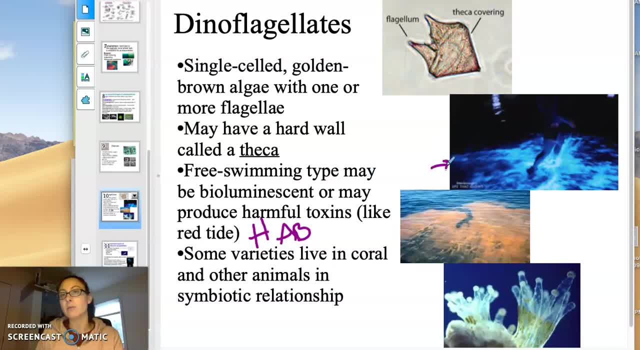 And so if you've ever gone to Puerto Rico or Mexico or certain parts of California, there are these free swimming ones, this totally different species, here, and as they get jostled around the water they glow. So this blue light is actually from dinoflagellates giving off a little. 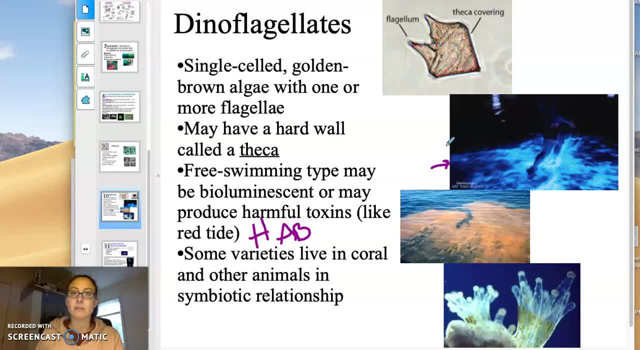 bit of bioluminescence. Other dinoflagellates live as symbiotic organisms inside of squid and other deep sea creatures. And finally there's a group of dinoflagellates that you can see here. All of these little dots in here are dinoflagellates that are called zooxanthellae, or zoox for short. 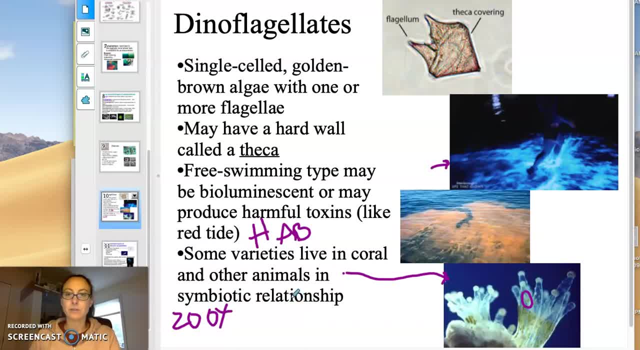 They produce the oxygen and sugars that corals and giant clams use, And so they're really important in marine ecosystems as being part of the food chain and being part of those sort of structural organisms. But it's a symbiosis, so you have one species living inside of another. 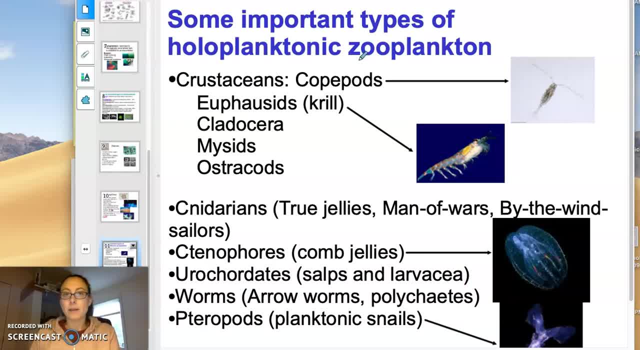 So when it comes to the zooplankton, I'm going to talk about the ones that live their whole lives there, and then briefly about some that only spend their larvae phase there. So here's a copepod. This is an actual light microscope photograph of one. They have these long antennae and they are able. 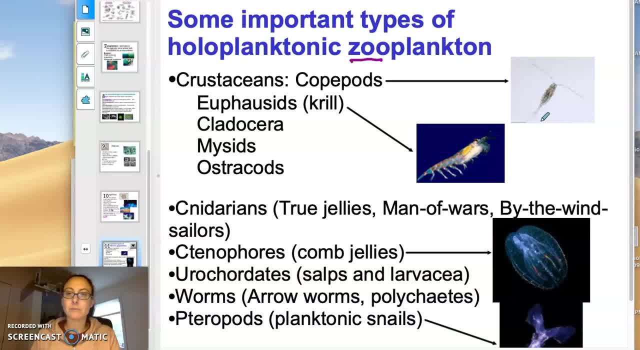 to swim around and some light sensing organs, So that's why sometimes you see them as having a big, giant eye there. This is the most abundant type of zooplankton out there. Krill, which you might have heard of before, is part of a group called euphausids. They look like this. They're very similar to mysis shrimp. 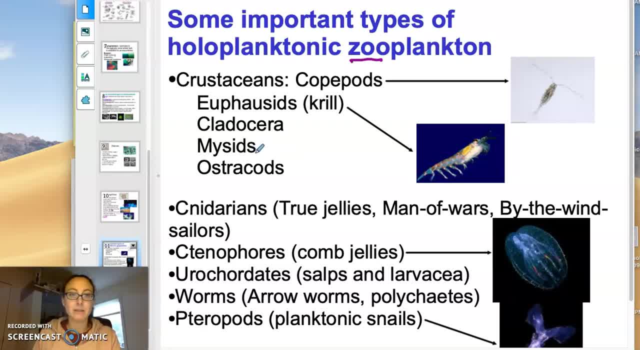 So if anybody keeps a fish tank and has to feed frozen mysis shrimp to their fish, this is kind of what you're doing. Very, very important for all those fish and whales and sharks that eat krill and other kinds of plankton. And then we have other things that don't have a hard shell. So 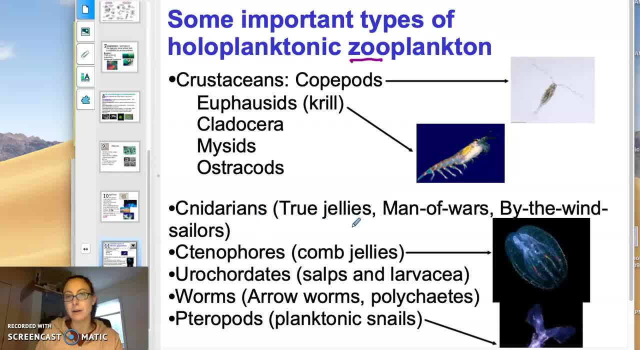 cnidarians, which are like jellyfish and man o' war, Portuguese man o' war. those have stinging cells related to them, or ctenophores or comb jellies that don't have any stinging cells And 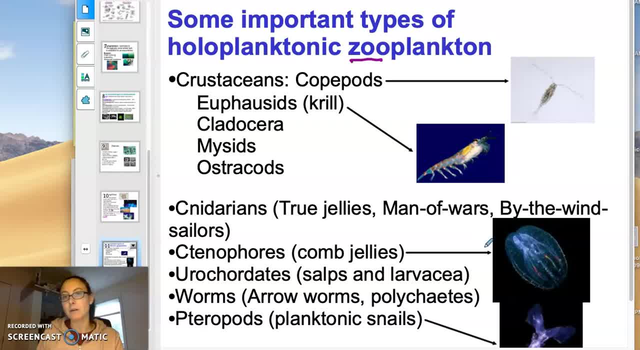 that's actually what a lot of people in Marion call moon jellies, but actually they're a ctenophore. They're not a moon jelly, So they're not a moon jelly. So they're not a moon jelly, So they're not. 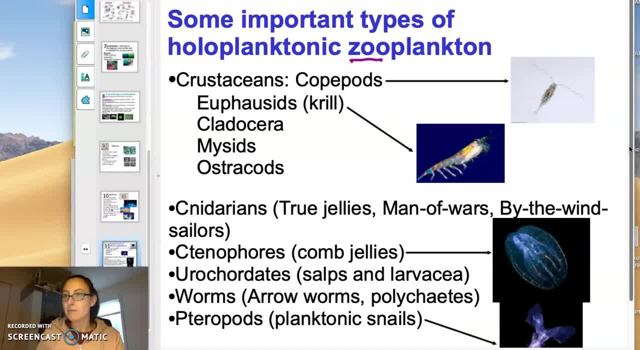 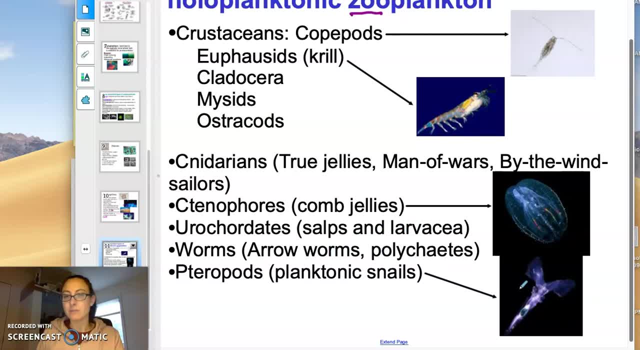 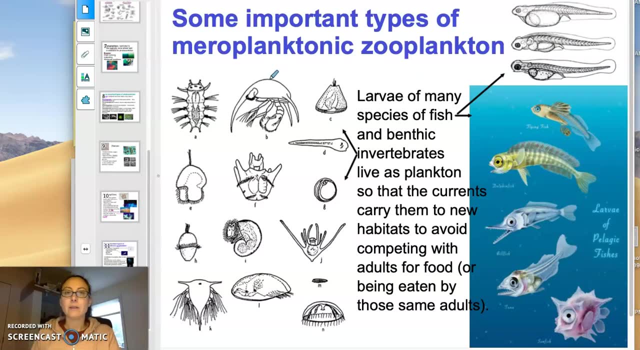